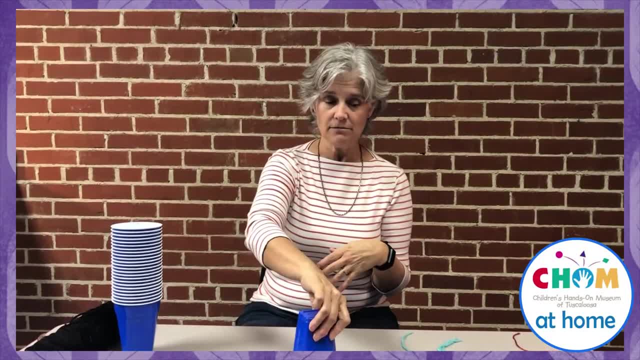 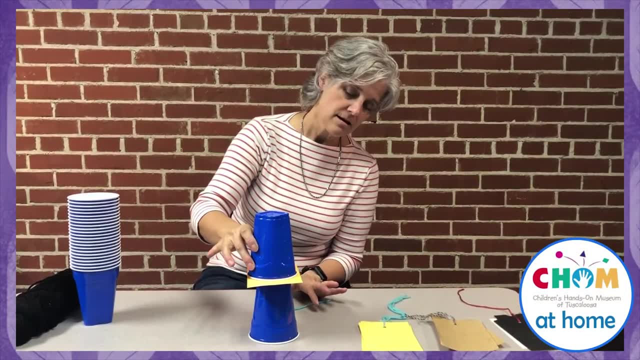 Now you can play around with this a little bit. You can stack in this direction, so we'll start that way. All right, so I'm going to use the plain, the plain paper first, All right, so here's what I need to do. Let me turn it that way. 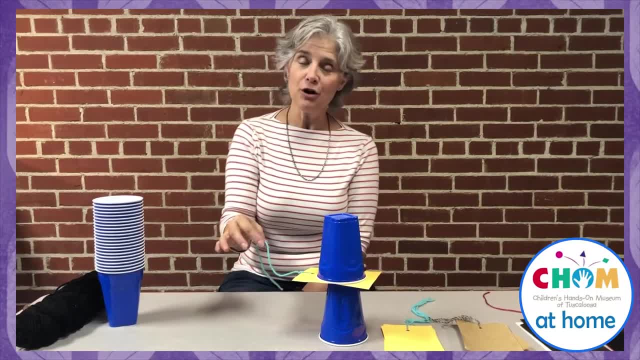 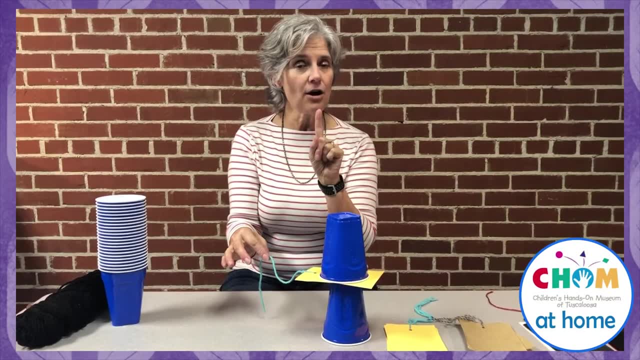 So you can see better. So here's what you're going to do: You're going to tug your yarn to pull the card out and because the card is smooth, friction is not going to hurt it and it's going to help it. just go straight down like this. So see, there was very little friction. 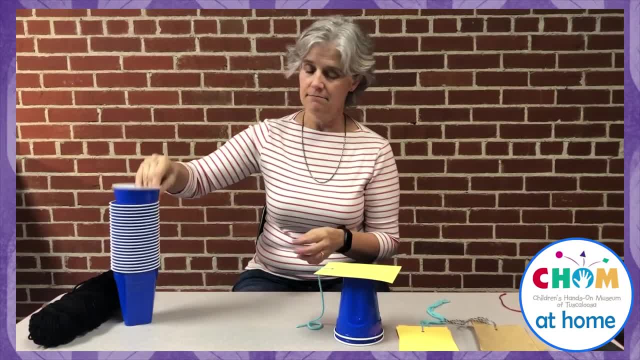 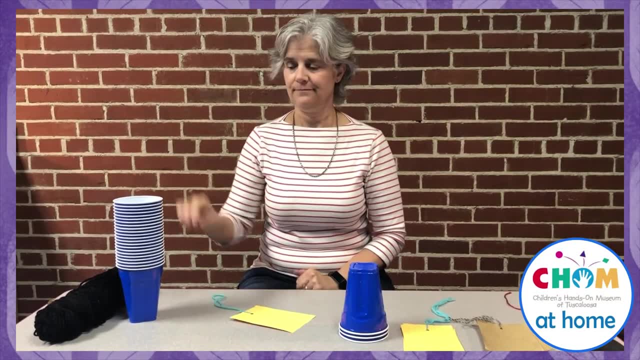 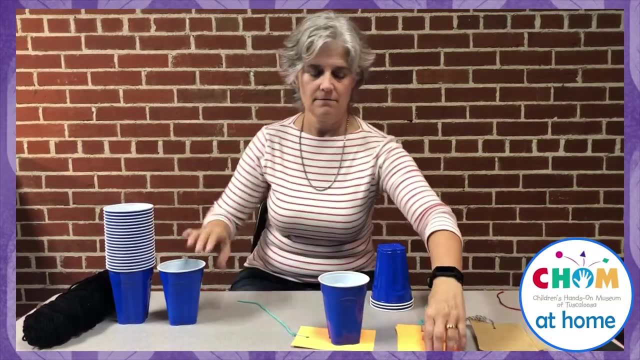 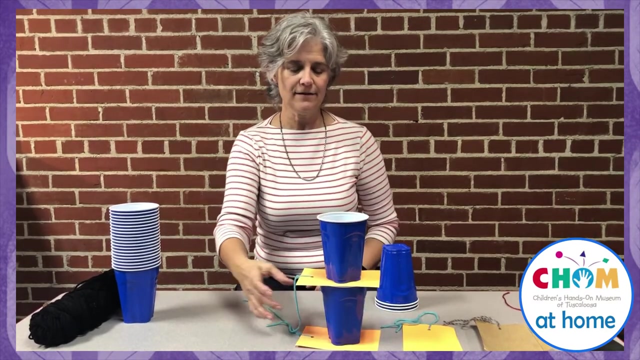 because the card is smooth. I can do it again. Perfect, All right, I can even turn them The other way. Oh, and let's put one down here too. This lark came up with that one. You just want to make sure they're lined up, and we're going to try this and see if it works too. 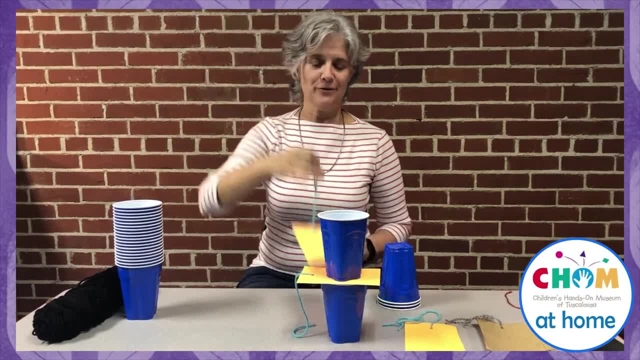 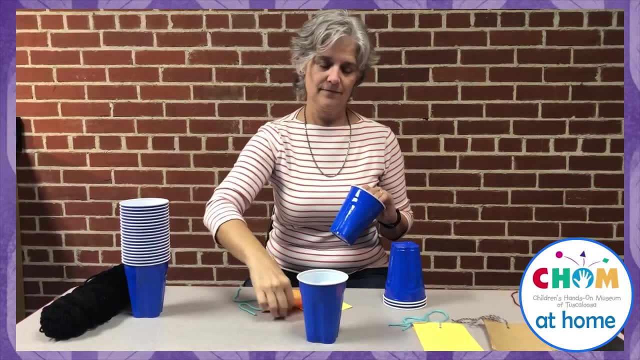 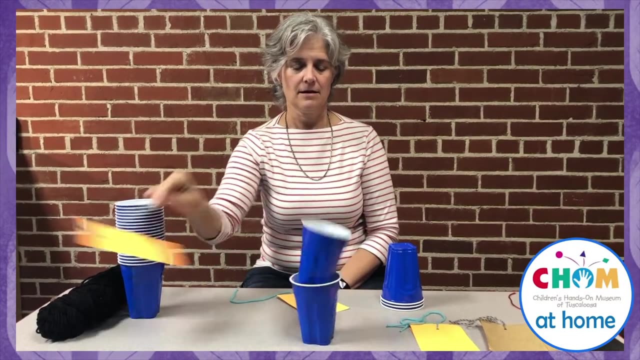 First, let's try this one. Look at, that Didn't move. All right, will they stack? Oh, they didn't. that time Let's try it again. I may not have had them stacked perfectly. All right, There we go. Okay, so this time I'm going to stack my cups and I'm going to use 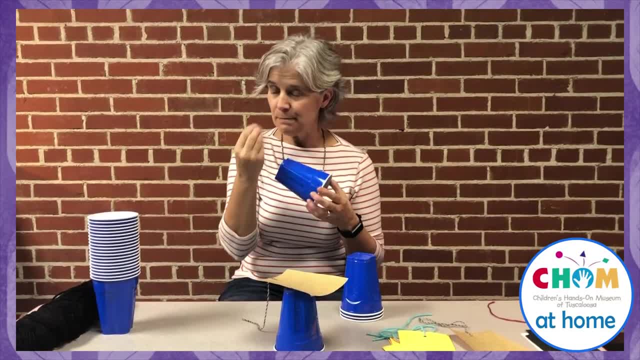 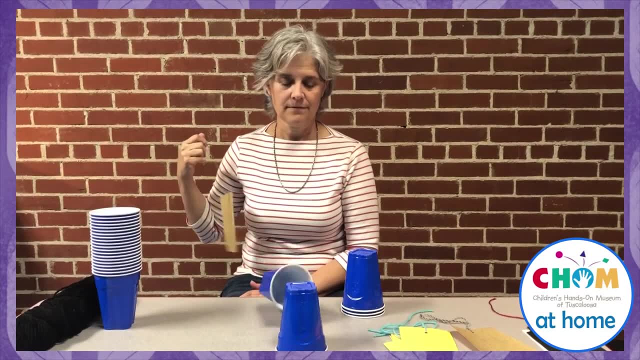 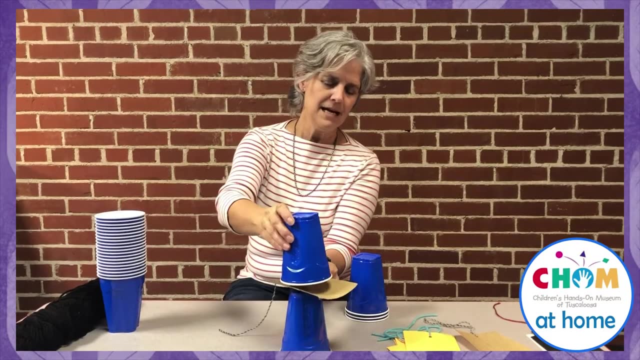 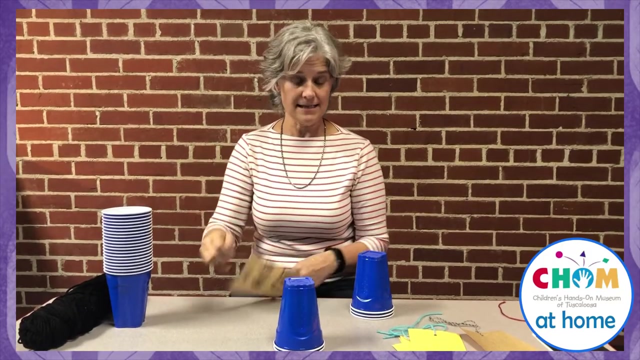 the sandpaper. The sandpaper is rougher, It's bumpy. Let's see what happens when I tug the yarn this time. Okay, let's try that again. Make sure you stack the cup right above the bottom cup. Oh, it worked that time, I'm not sure why. Let's try the other direction. 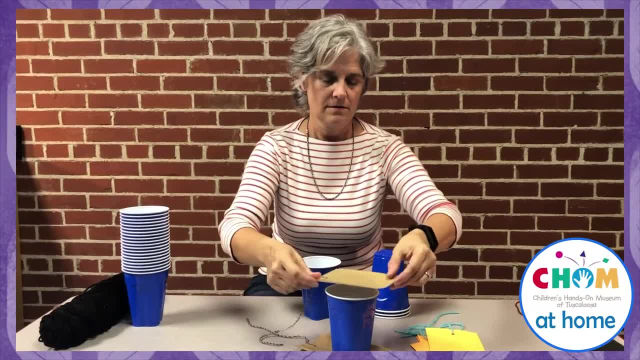 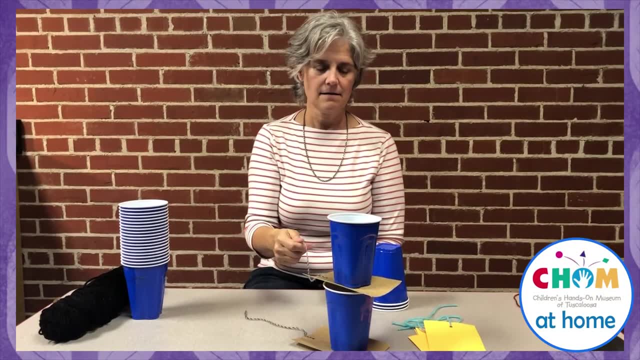 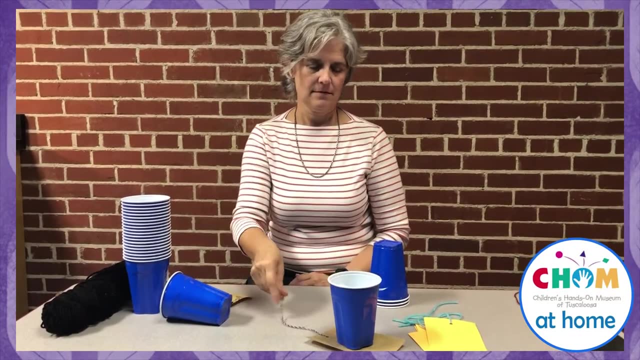 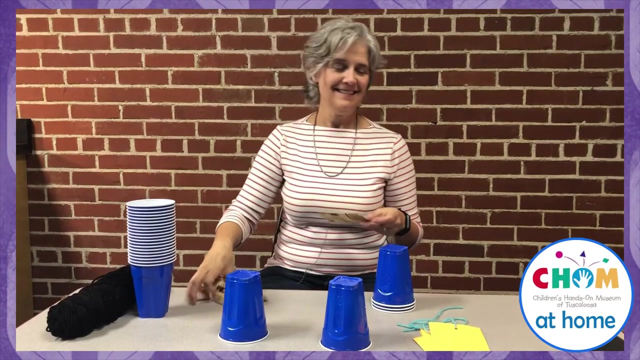 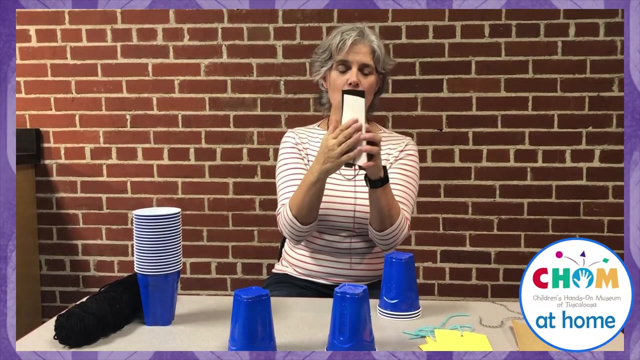 I do have two. You can kind of see that it's not flat. I don't know if that's affecting it. All right, all right. so with our super duper sandpaper we put a plain card on the back of it.